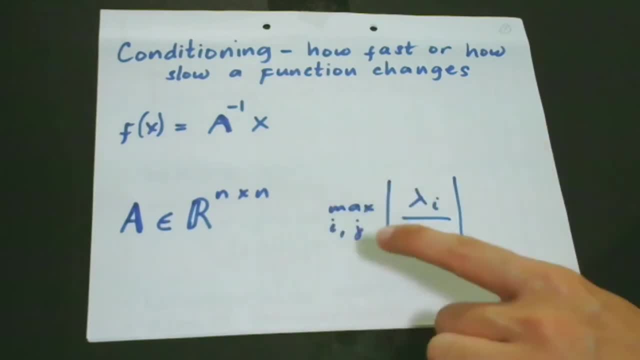 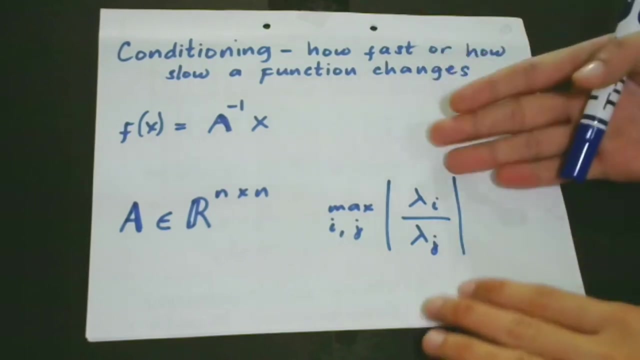 and it has an eigenvalue decomposition and its condition knowledge is a function of A number is computed by dividing eigenvalue i and eigenvalue j, So this means that the condition number is the ratio of the smallest and the largest eigenvalue. So anyway, if 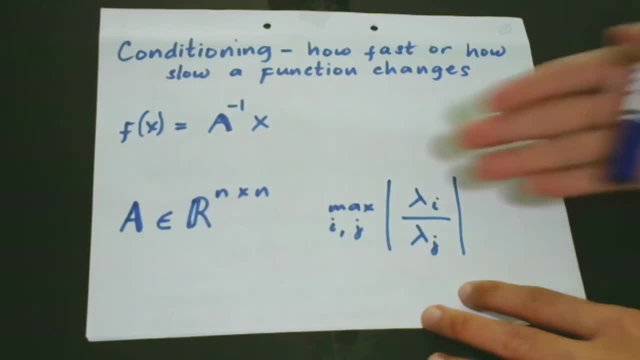 you would like to know more about decomposition, because decomposition is an important part of this lesson. I have a lesson about that, So the link is given in the description below and please you watch it for you to be able to understand what I am talking. So you may. 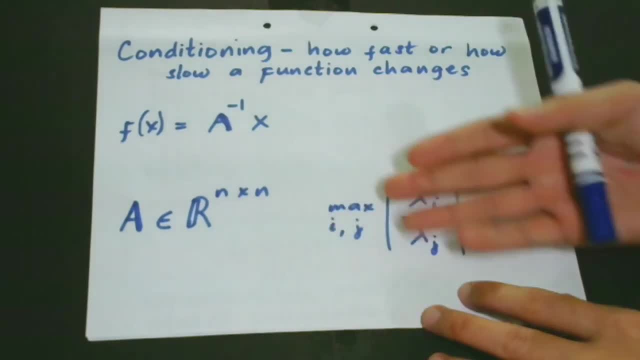 pause this video for a while and come back if you're done with decomposition. So what does this mean? By intuition, the condition number of a matrix is how close a certain matrix to being singular, un-invertible- Let me write that here- Singular. 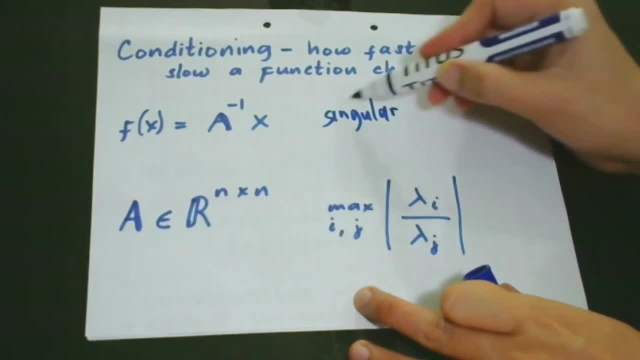 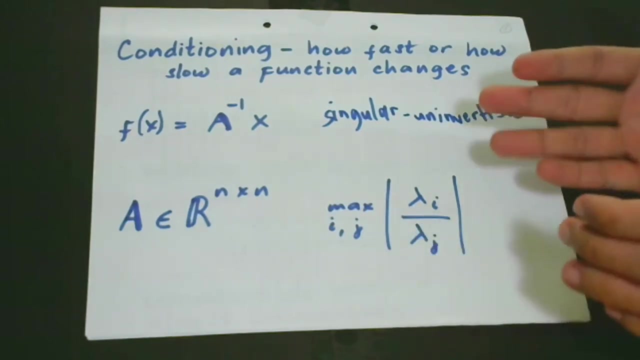 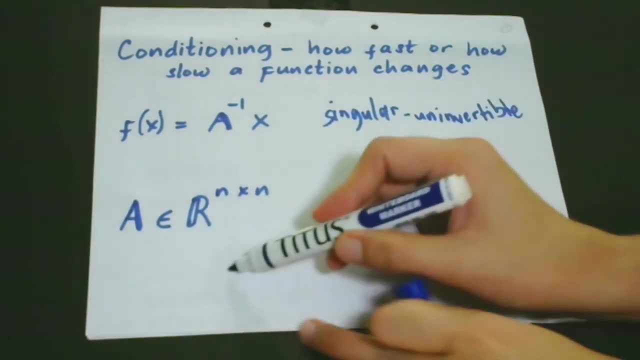 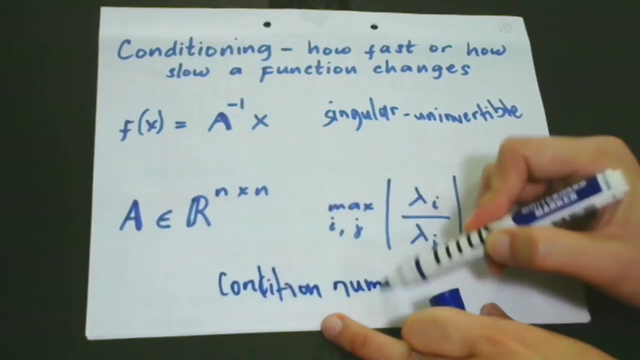 un-invertible. So what do we mean when we say singular un-invertible? So this is actually a row and it does not have any inverse. So then, what is the essence of this condition number? Okay, I think I have to write here condition number. So condition number Why. 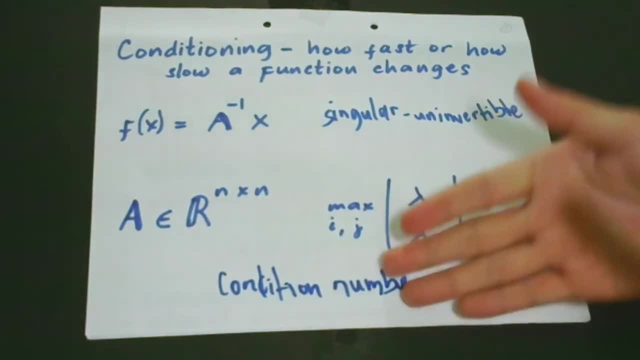 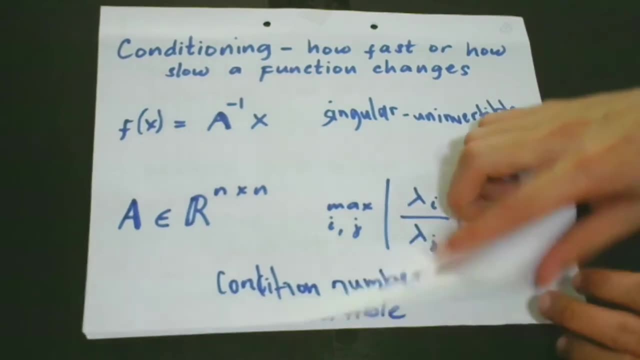 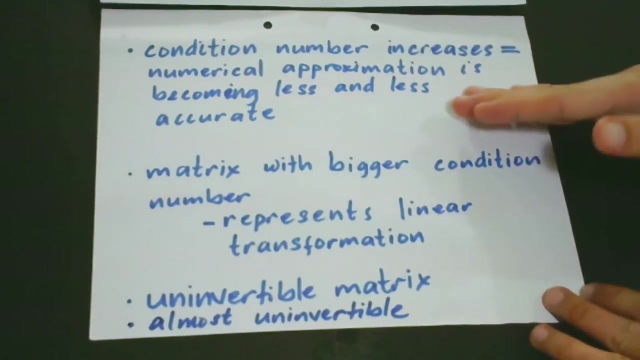 do we have to know this condition number? So what, then, is the essence of a condition number? So when the condition number increases, let's go to okay again. when the condition number increases, numerical approximation is or numerical approximation. algorithms involving matrix inversion is becoming less. 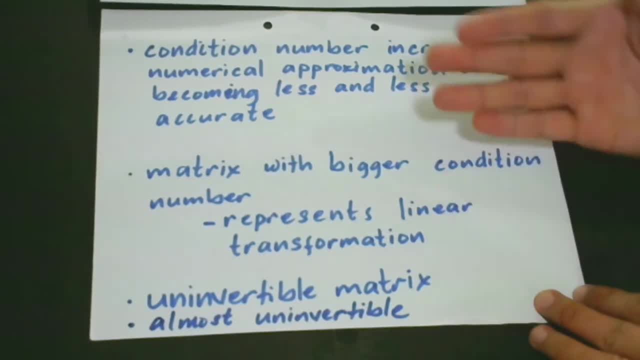 and less accurate. So what's next? What's going to happen if this is the case? So when this happens, it becomes sensitive to error The input. So remember our lessons before about the rounding off or the rounding error. So I have that in lesson number 16.. So please study the two errors: the overflow and the. 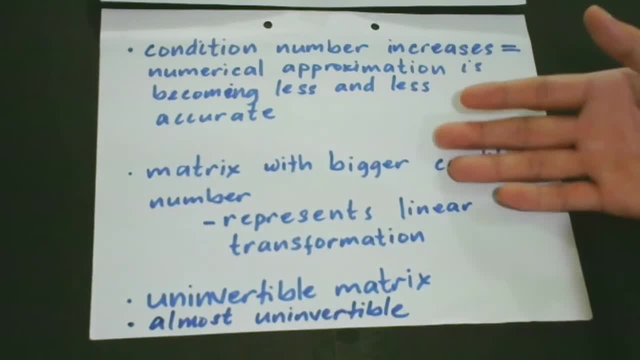 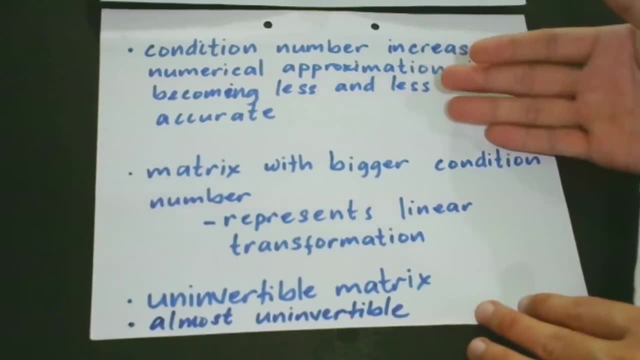 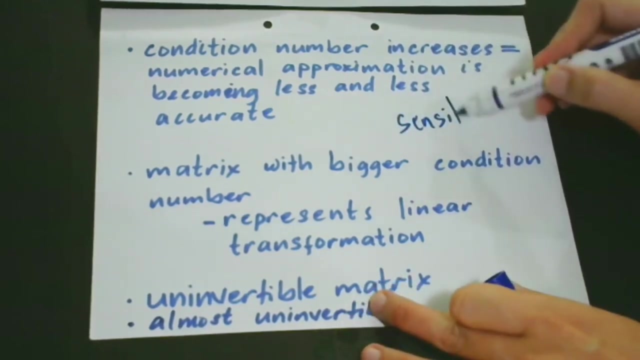 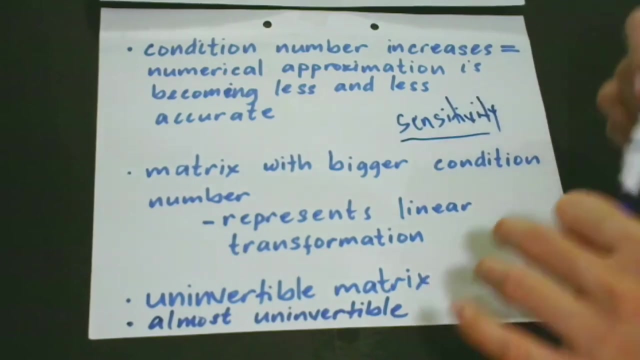 underflow, because that is also an important part of this lesson. So I would like to point out that this sensitivity is an intrinsic property of the matrix. Let me write here sensitivity. Okay. so, as you could see, as we sensitivity, as we go along with our discussions, with our lessons in this. 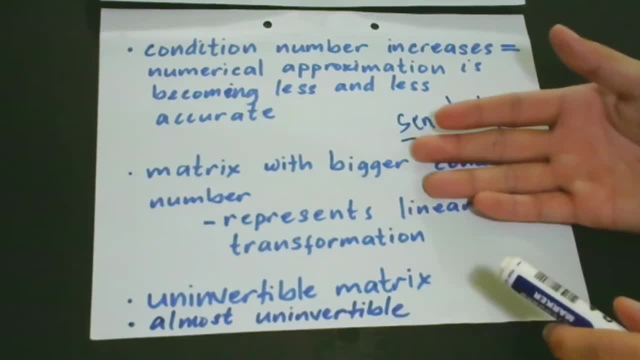 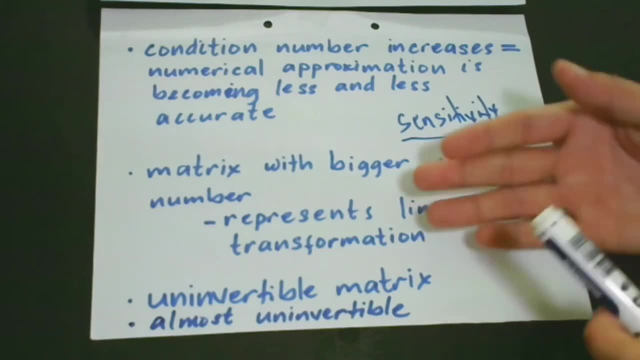 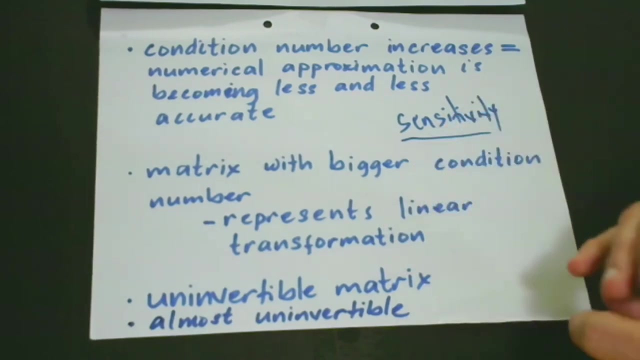 course we are meeting lots of terms which I think you have to familiarize, if not memorize all of them, because that is really very important, especially if you would like to major a major machine learning engineering. so it's really very important. so again, I would 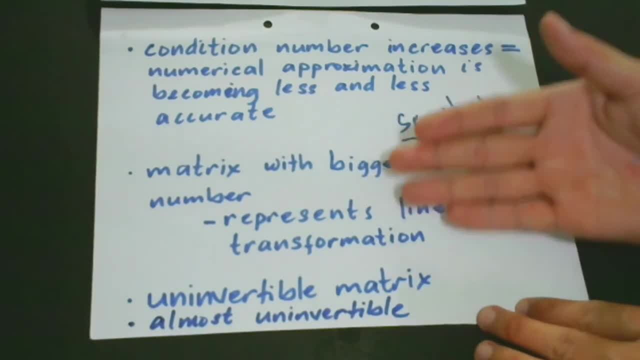 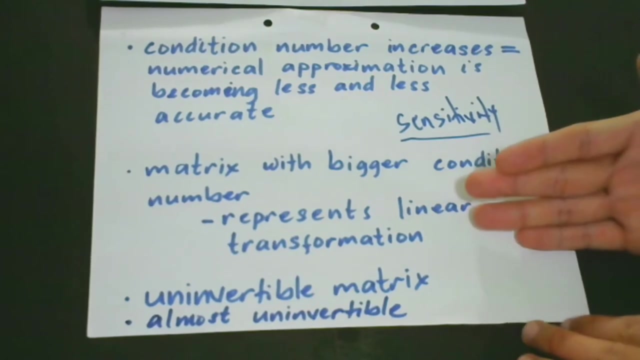 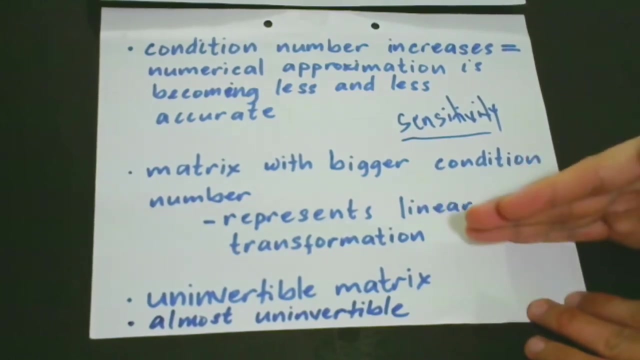 like to point out that this sensitivity is an intrinsic property of the matrix itself and not because of other outside phenomena like the rounding hour doing matrix inversion. okay, so examining a matrix with bigger, with bigger condition number, we can say that it represents linear transformation. so between vector, 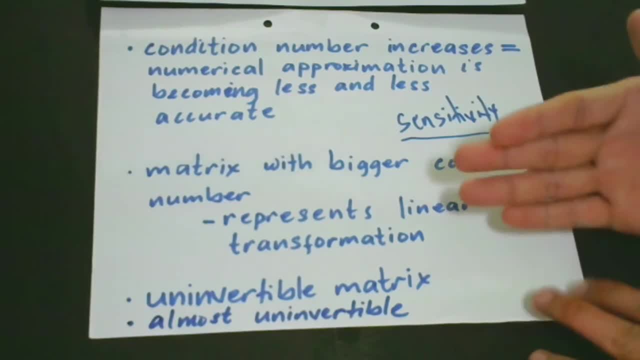 spaces. so it means that when there is perturbations in the input, even the smallest deviation, an impact is created in the norm of the output vector. so I know that you do not want this to happen, right, of course, whoever would like to have a problem, I think something is wrong because in this case, if, if an 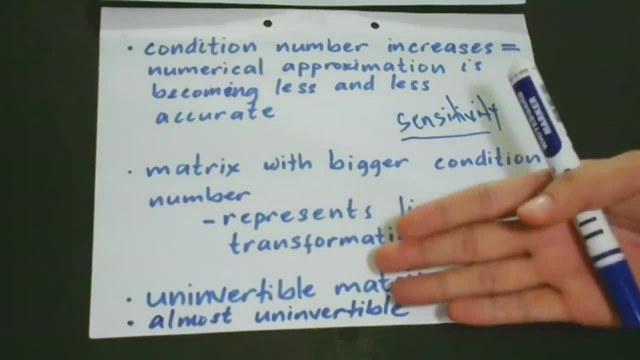 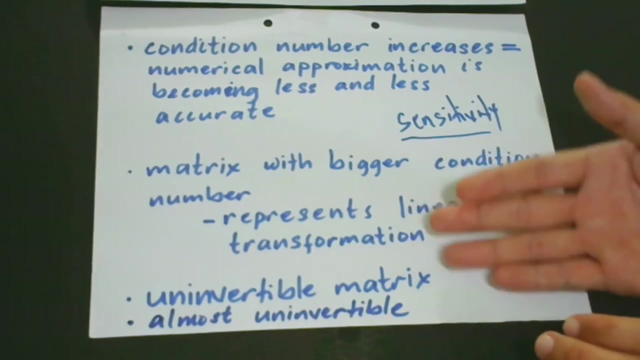 impact is not what is really normal, then something is wrong with our data. later we will have that, so it causes a problem for the purpose of scientific computation. so there would be rounding errors in the inputs, which or which can result to large changes in the outputs. okay, so 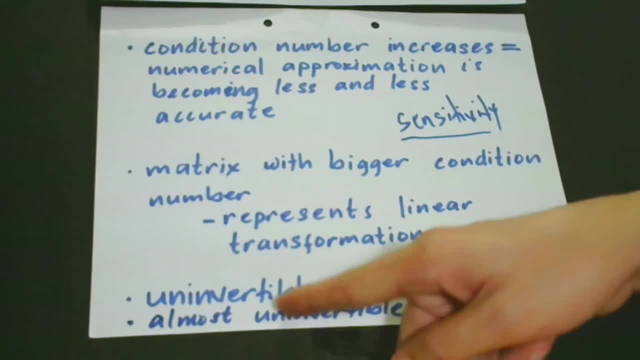 when our output is an, an invertible matrix. basically, it becomes useless. so maybe you would like to ask: why is it that it becomes useless? well, the answer is that is that at any point, we cannot make interpretations with respect to any of those lower dimensional features. so the bottom line here is that the choice 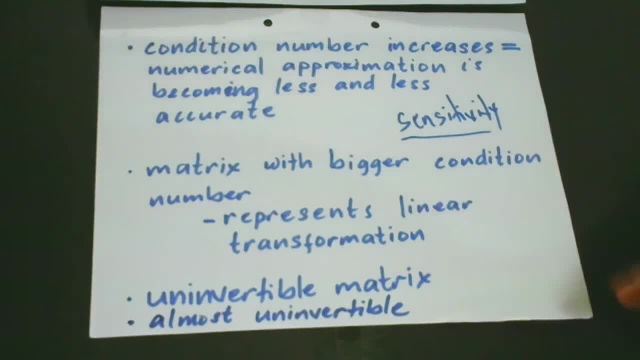 of a particular value of that metric can be used in another convenience. if we are, representation becomes arbitrary. let me write here: arbitrary, okay, your choice of a certain representation. again it becomes arbitrary. so maybe you would like to ask me, joseph, why is it that at this point it becomes arbitrary? okay, so this is so because you do not have enough data to arrive. 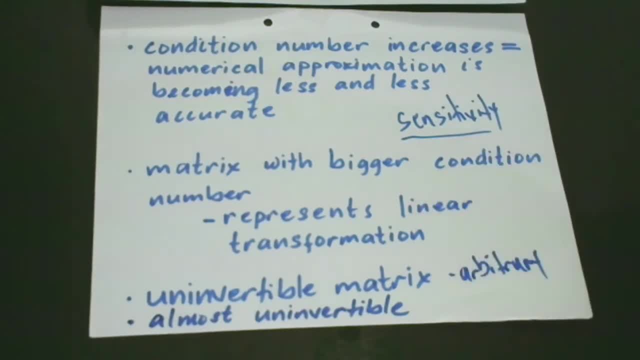 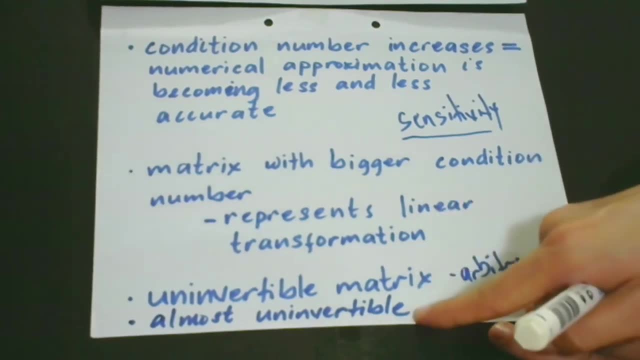 at certain representations. so what if the output matrix is almost uninvertible? again here is uninvertible, here is almost uninvertible. what is the situation? what will happen? so if our output matrix is almost uninvertible? this happens when a matrix has a certain 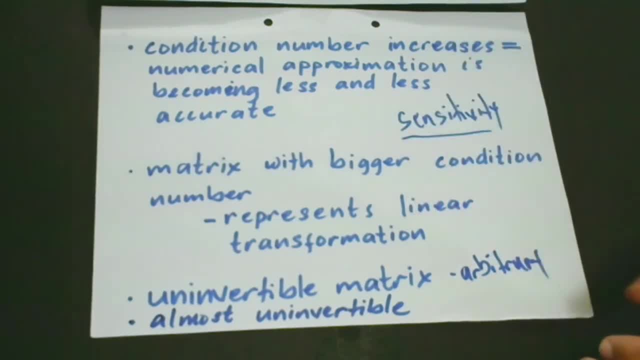 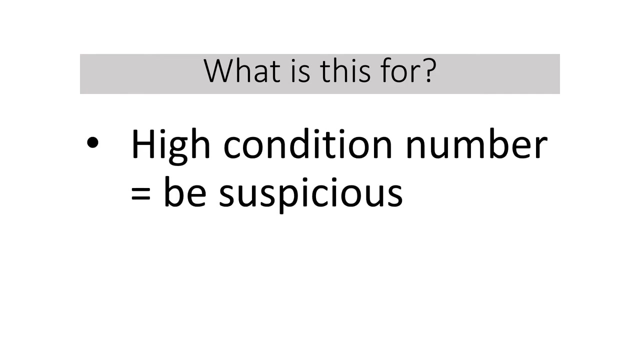 condition number. okay. so it essentially means that numerical condition algorithms get less accurate. so when it becomes less accurate, then of course something is really wrong and you have to investigate. what is this for? why do we have to study this? if your algorithm gives you a high condition number, then it is time to be suspicious. 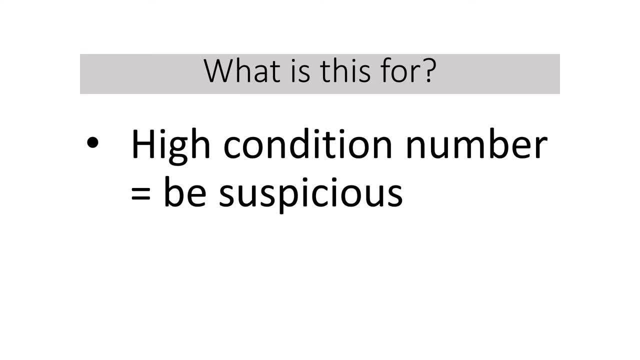 investigate, but be cautious. what you have to do is that you're going to track non-optimal solutions that are also close to optimal one, so better. yet if you compare them, if they are all similar, then it means that you can still simplify more your representation. if there is no point of